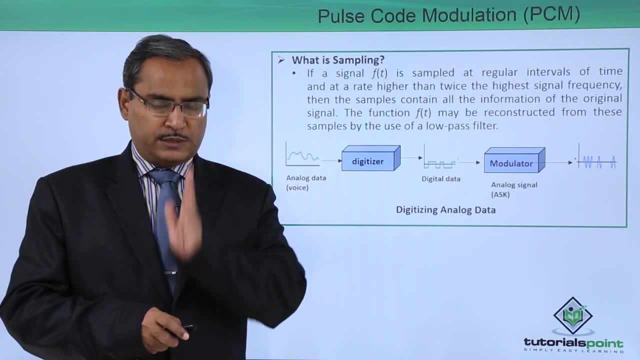 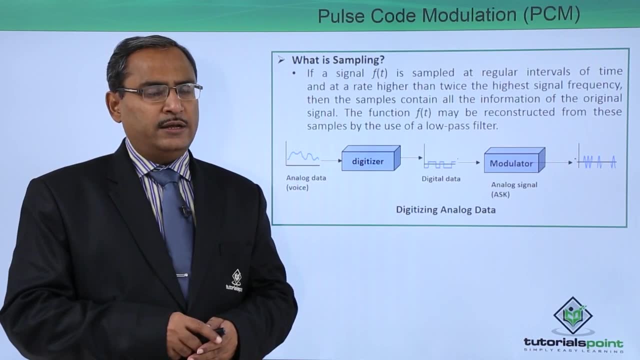 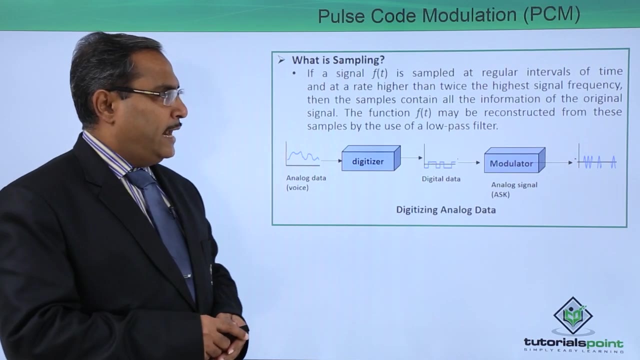 maximum frequency of the analog signal, So that we also can go for the respective sampling, and from the sampling we shall get the respective digital signal and later at the receiving end we shall convert it to the analog data back again. So if a signal f of t is sampled, 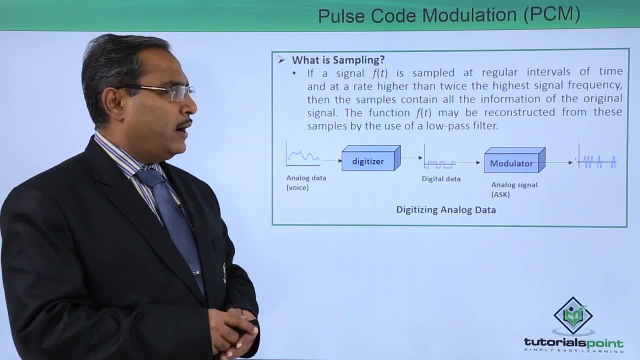 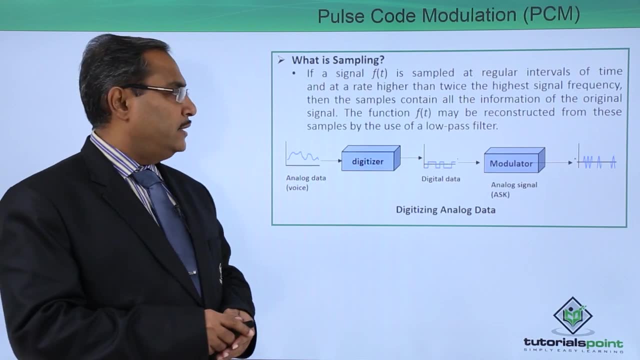 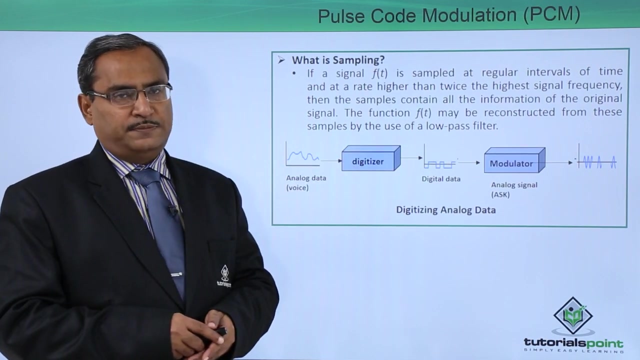 at a regular intervals of time and at a rate higher than the twice the highest signal frequency. then the samples contain all the information of the original signal. The function f of t may be reconstructed from these samples by the use of low pass filter. So at the 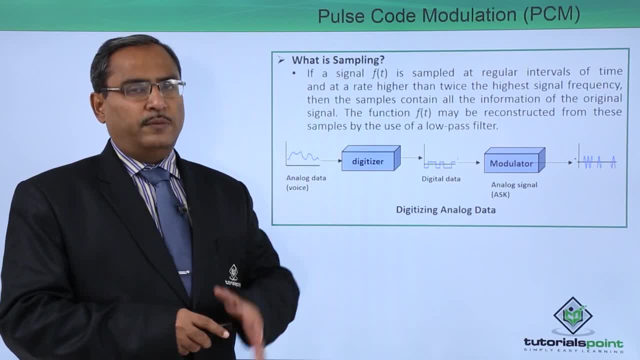 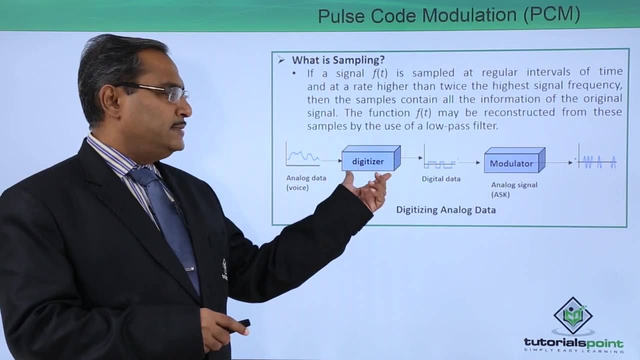 receiving end. from this sampled output, we can reform the analog data back again. So now this is our analog data. Let it be a voice Digitizer will convert it to the corresponding digital data. and then analog analog, that is ASK. analog signal, that is. 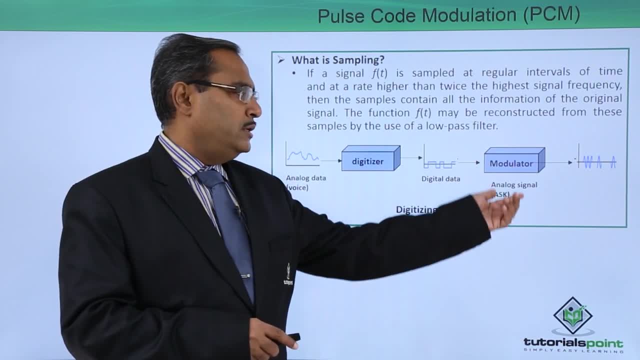 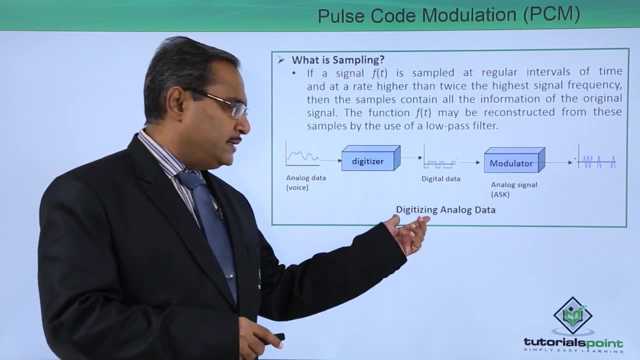 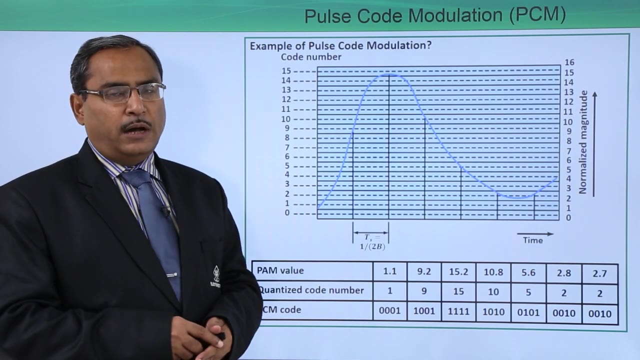 we are using some analog signal modulation technique, So one modulation So later- suppose it is ASK- and then we are going to back our analog data back again. So digitizing analog data will have the following steps. Now let us discuss the PCM. that is a pulse. 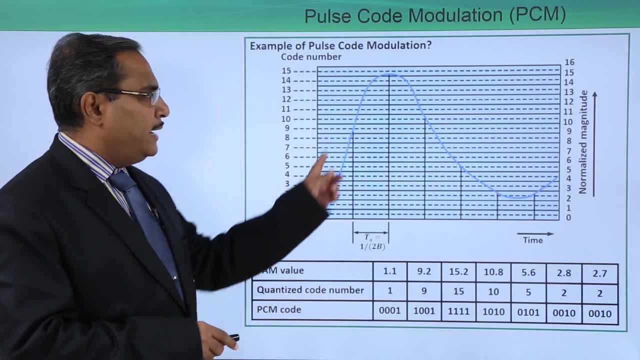 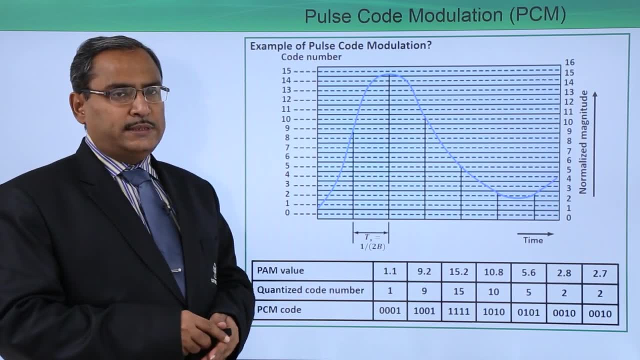 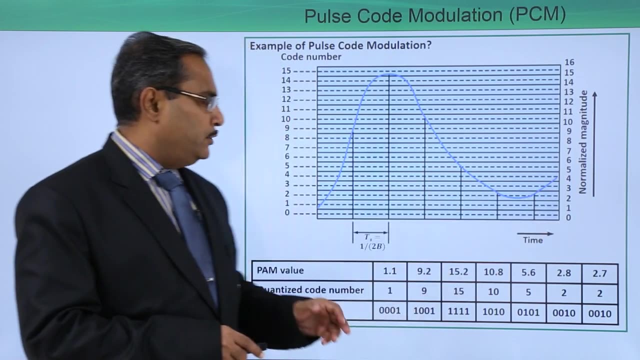 code modulation. What will happen? You can see that there is one analog signal we are having. This is our analog data, rather not signal analog data, and this particular analog data will be sampled at a regular time interval. So when we did the sample here, just look at this respective normalized magnitudes. 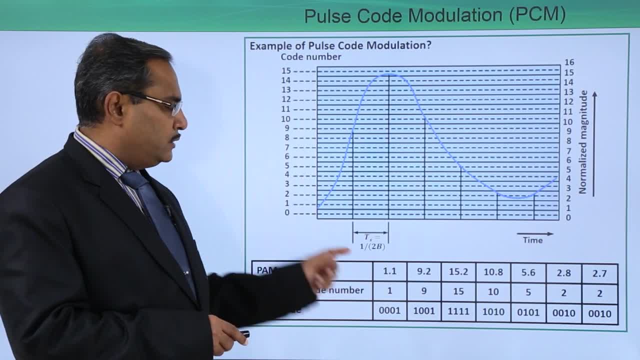 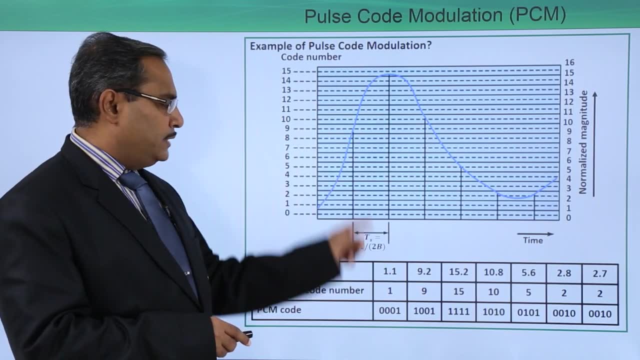 So when we sampled here, then this analog value was 1.1.. This is a PAM value, This is a 1.1.. Then here this particular PAM value is 9.2.. Then here this particular PAM value. 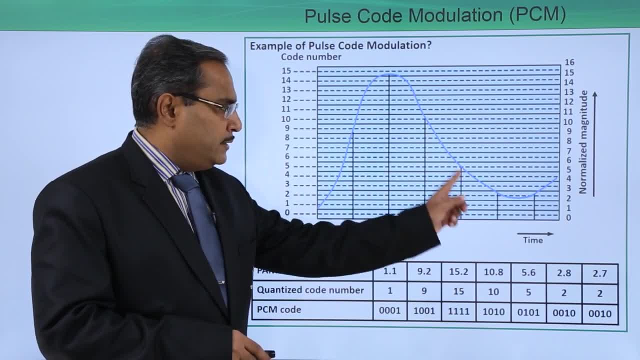 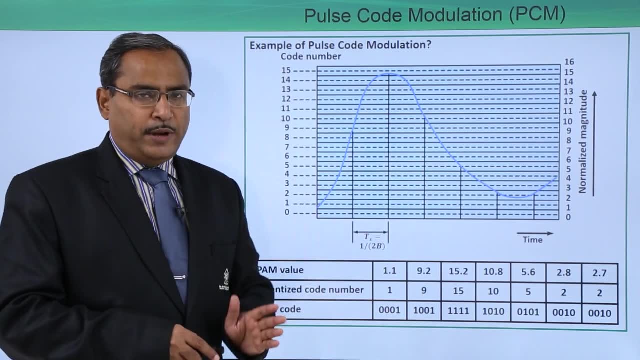 you can consider that one that is 15.2,, then 10.8,, then 5.6,, 2.8 and then 2.7, and so on. In this way we have, we have done the sampling, So we have done the sampling at regular time interval, and here the time interval is t? s. 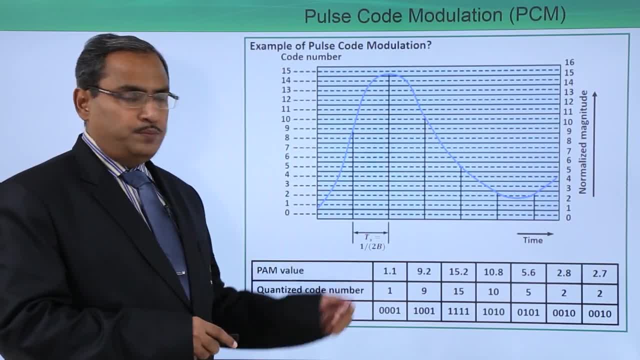 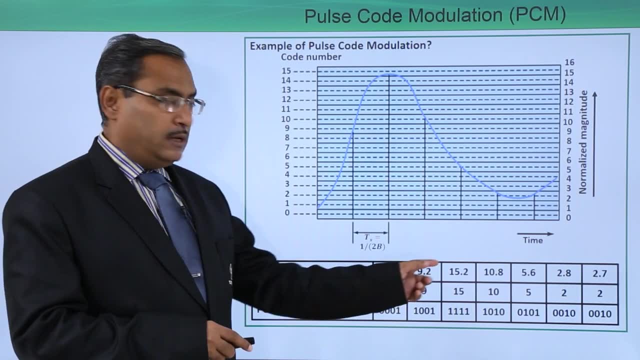 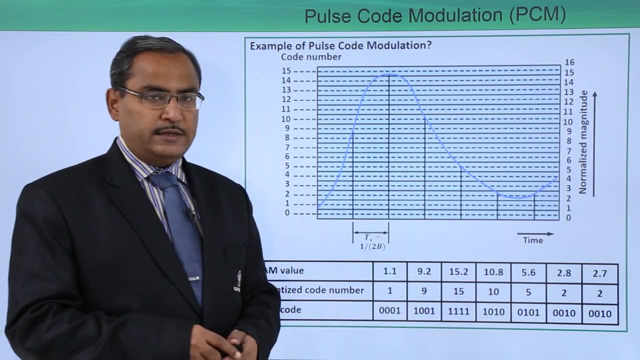 that is the time slice and that is 1 by 2 b. So now we are going for this quantized code number. So what will happen From this respective voltages? we are going to convert it to the nearest integer value. You can find that we have converted to the nearest integer. 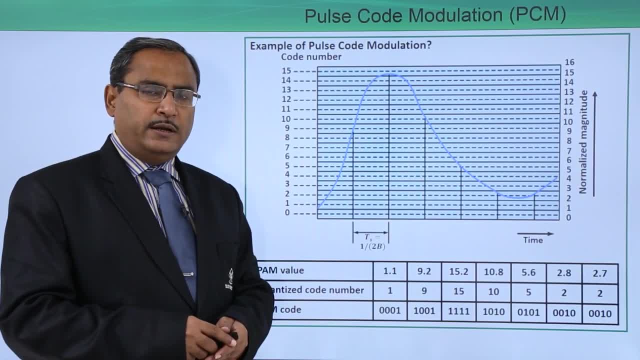 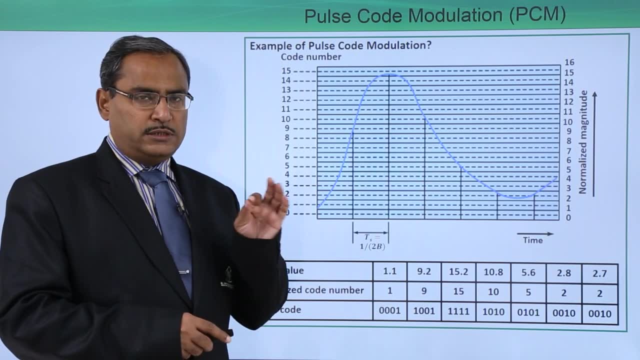 value. So what is the maximum value here? 15.. How many bits will be required to represent 15?? 4 bits, How 15.. Because 1 1 1, 1, if you consider 1, 4 times 1, 1 1, 1, that is a, if you consider this one. 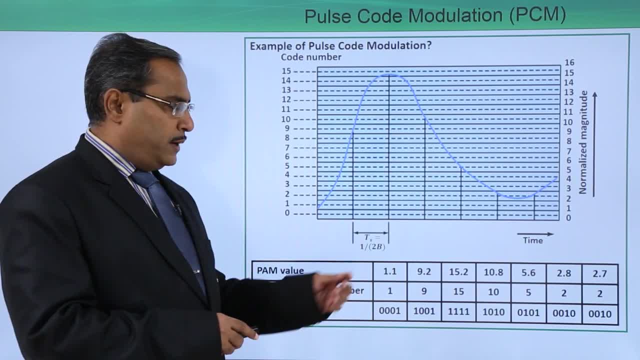 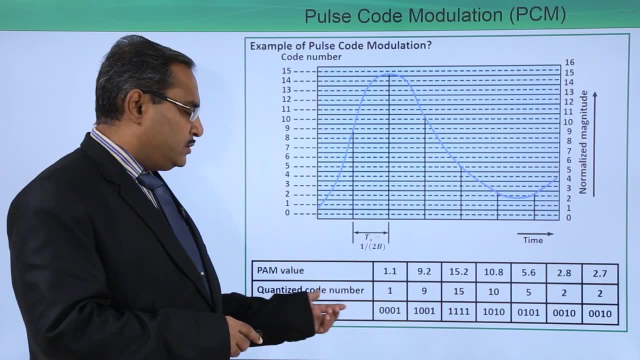 as binary, then it is representing 15.. So that is why 15 is the maximum value, and you can represent 15 by 4 bits. So all these respective, all these respective quantized code numbers are to be converted to the 4 bit form. So here we are having, that is 0. 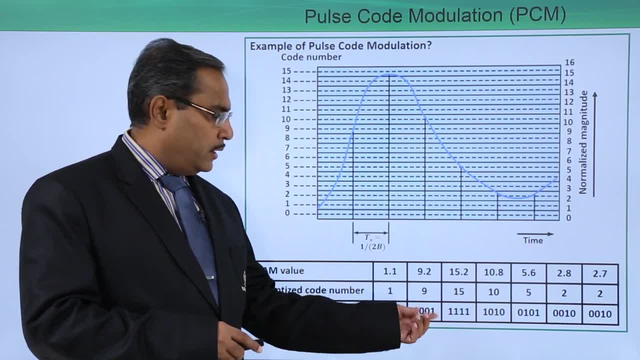 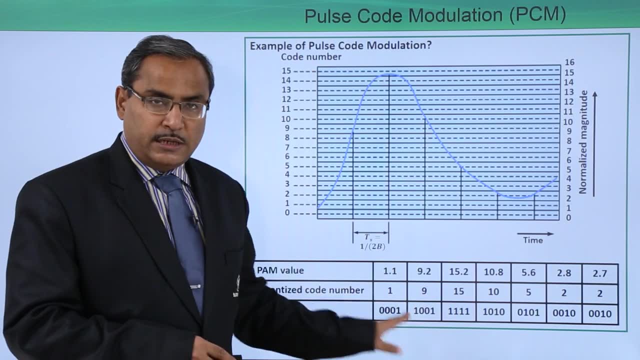 0 0, 1.. Why? Because it is 1, it is 9.. So 1 0 0, 1, it is 15, 1 1, 1, 1.. In this way we did the rest. Then what will happen? We shall send this bits, bits, stream of bits through. 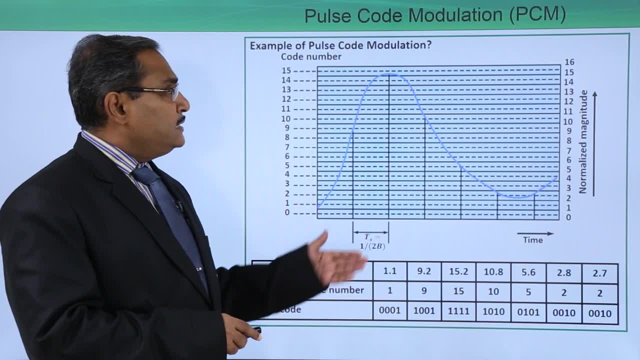 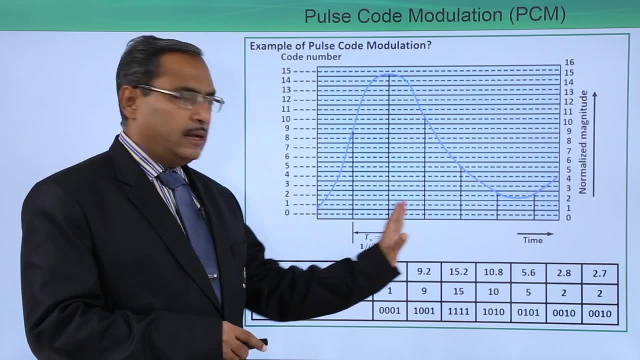 the media to the receiving end. So this is our pulse code modulation. So here we are going to take the frequencies. sorry, we are going to take the respective sampling after regular time interval and this is our T s is the respective sampling time. 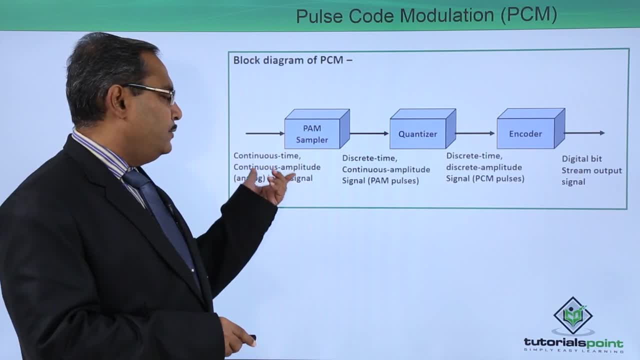 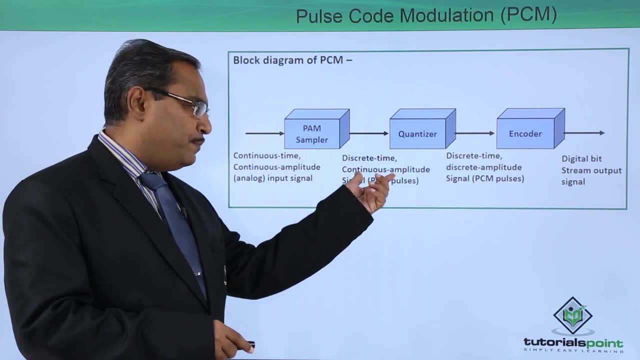 So what are the steps we are having? At first, we are having continuous time, continuous amplitude, analog input signal. Then we are having- this is the PAM sample- We are having discrete time, continuous amplitude signal, that is, the PAM pulses. 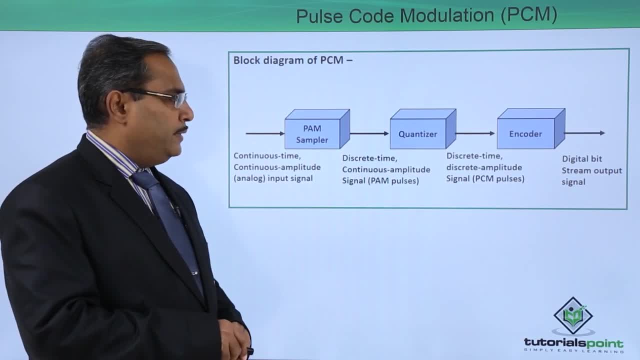 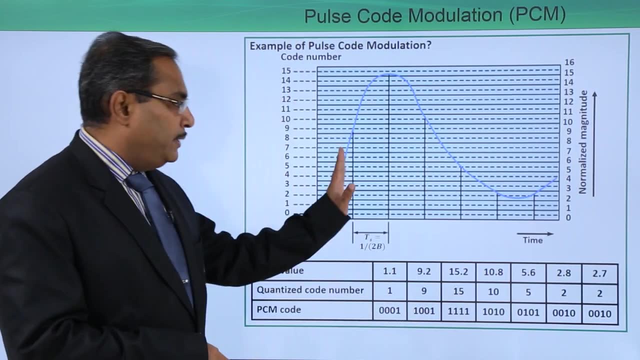 Why we are considering is that continuous amplitude. why? Because you can find that in the previous diagram also, we got this one in the fractions, So it is continuous, but we are having the discrete observation, So that is why we can call it as discrete. 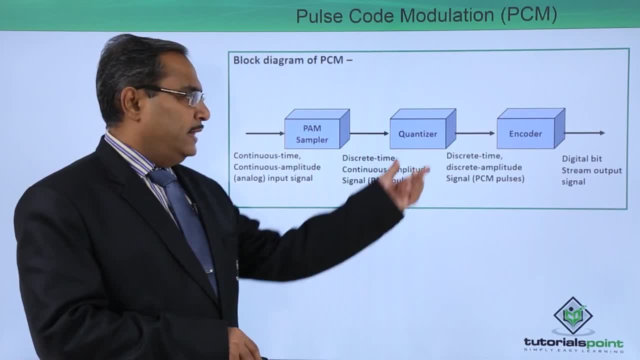 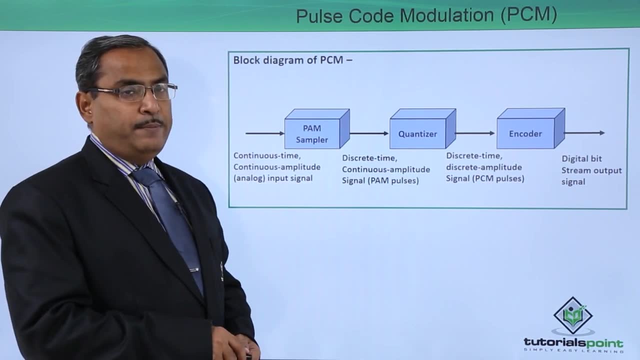 time, continuous amplitude signal, that is, PAM signals, and then quantizer will come into the scene and we will be having discrete time, discrete amplitude signal. that is our p, c, m pulses. why we are considering this one as discrete time, discrete amplitude, because 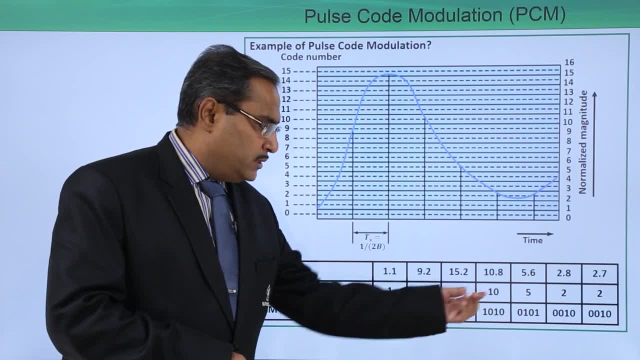 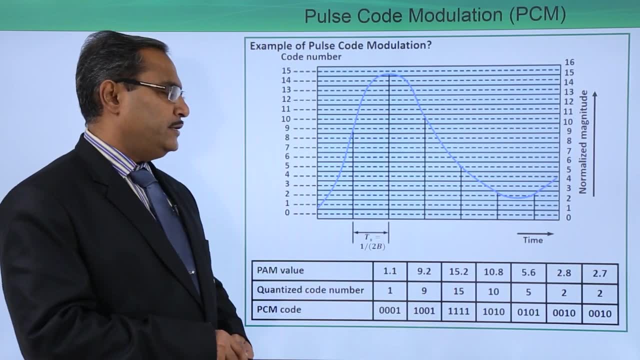 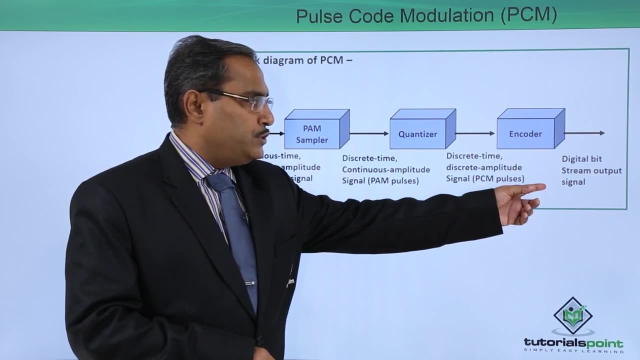 you can find that we are making them quantized, So they are discrete. that cannot be any value in between 9 and 10, either 9 or 10.. So that is why the values are discrete in nature. and then we are having this encoder at the receiving end for the digital bit stream output signals.